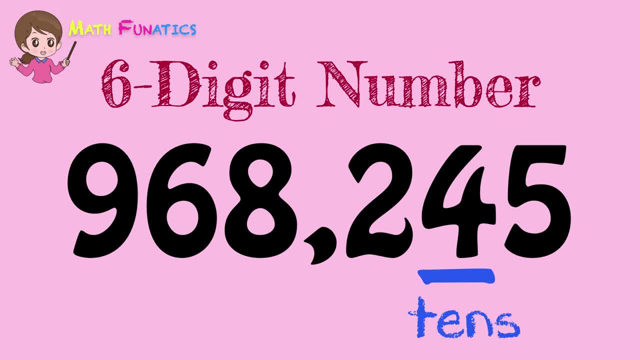 1's, 10's, 100's. How about the next digit, which is 8?? 8 is in the 1,000's place. Next is 6, which is in the 10,000's place. Finally, 9 is in the 100,000's place. 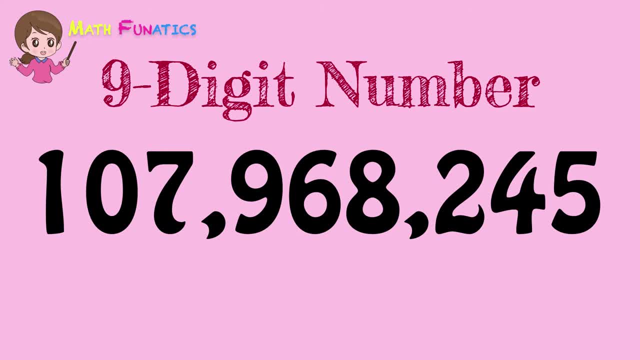 Let's add more digits to this number. Let's add more digits to this number and make it into a nine-digit number. Again, let's identify the place values, starting with the rightmost digit. Say them together with me: 1's, 10's, 100's, 1000's, 10,000's, 100,000's. 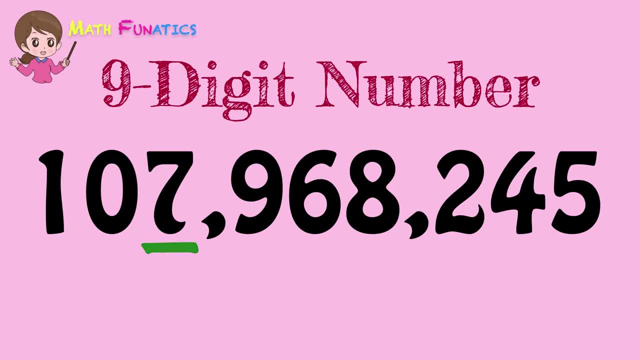 How about the next digit, which is 7?? 7 is in the million's place, The next digit, which is 0, is in the 10 million's place And, finally, 1 is in the 100,000 million's place. 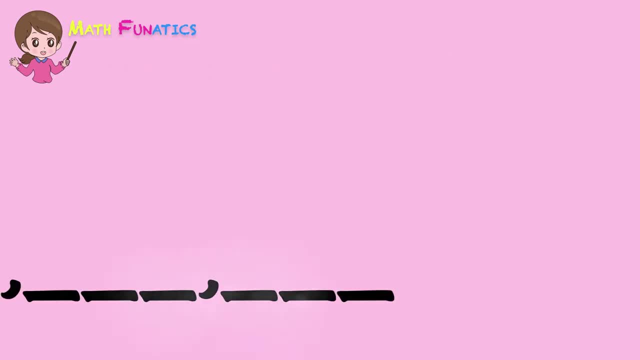 This time, let us list down the different place values that we've learned. So we have the 1's, 10's, 100's, 1000's, 10,000's, 100,000's. So we have the 1's, 10's, 100's, 1000's, 10,000's, 100,000's, 1000's, 100,000's, 10,000's, 100,000's. 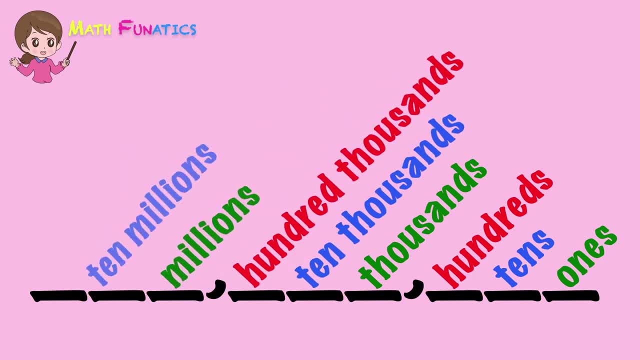 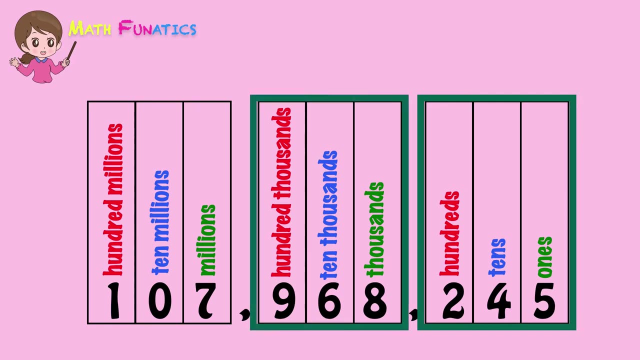 thousands, millions, ten millions and hundred millions. to know further about these place values, let's put them in a chart. in this chart, the digits of the whole number are grouped into threes. each group of three digits is called a period. a space or a comma is used to separate periods. the first period is: 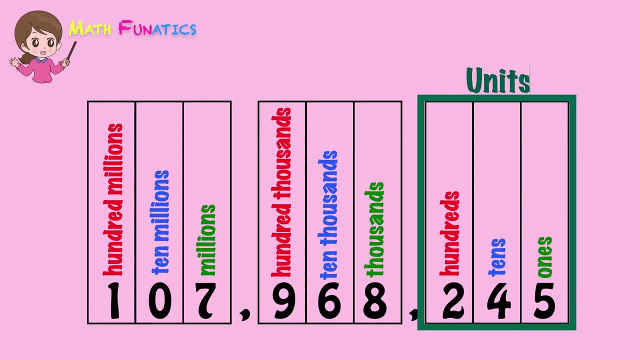 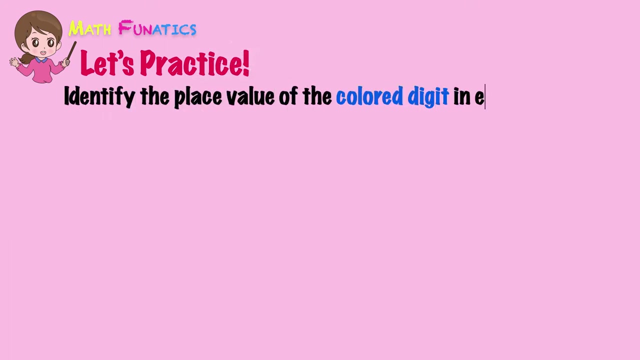 called the unit's period, the second is the thousands period and the third is the millions period. billions is the next period after millions. just like the other period, billions has also three places. now let's practice what you've learned with these examples: identify the place value of the color digit in each number: the color.